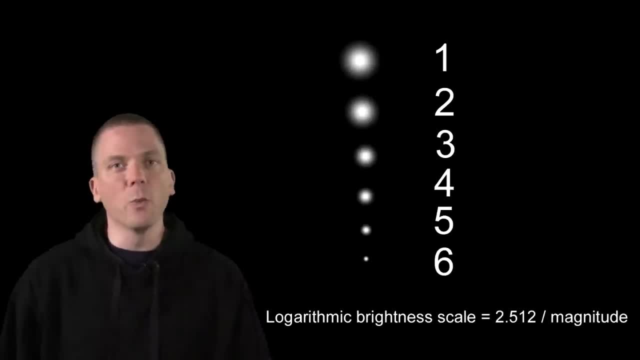 scale that meant that the brightest stars were 100 times brighter than the dimmest. It also allows for a fairly easy way to determine other brightness differences. The difference from 1st to 3rd magnitude is 6.3 times 1st. 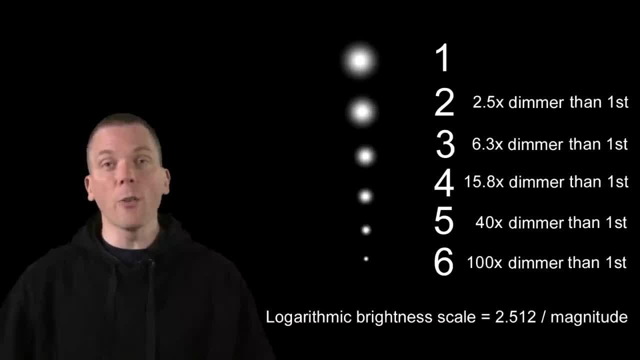 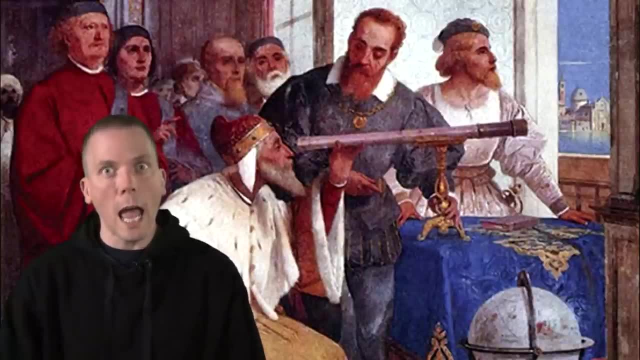 to 4th, 15.8,, 1st to 5th- about 40 times. This worked just fine until Galileo turned a telescope towards the heavens and humans discovered there were a lot more stars out there than just the 1st through 6th magnitude. 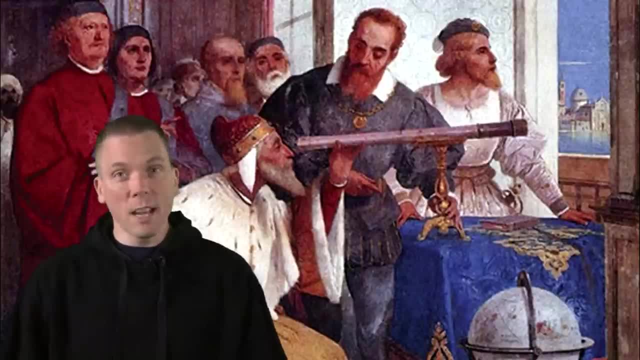 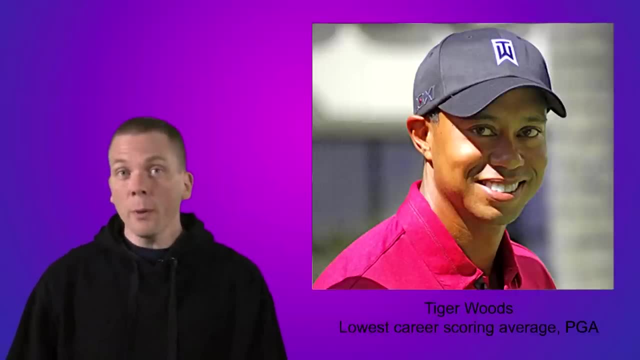 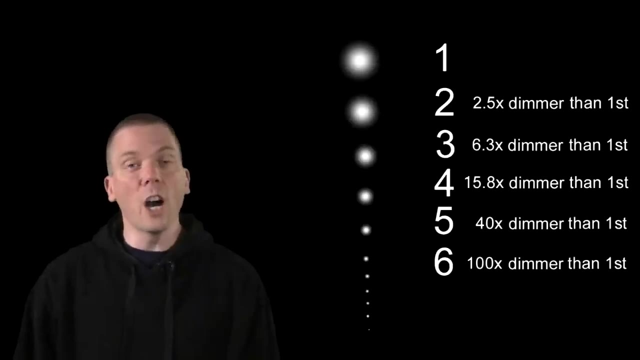 ones that they could see naked eye. But what they did was just extrapolate that scale further, So much like golf or ERA in baseball: the lower the number, the brighter the star, and the higher the number, the dimmer the star. 11th magnitude is 100 times dimmer than 6th. 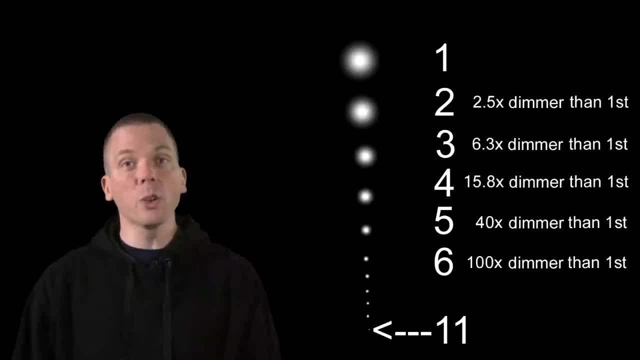 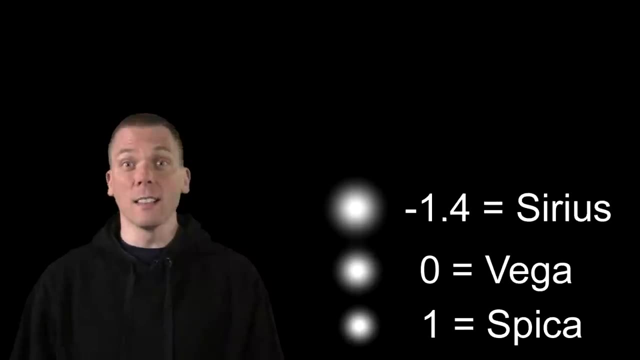 magnitude, And that 11th magnitude star would also be 10,000 times dimmer than a 1st magnitude star. In the other direction we have some objects that are brighter than 1st magnitude stars. Hipparchus actually fudged the numbers a bit. The star Sirius in the winter sky is definitely 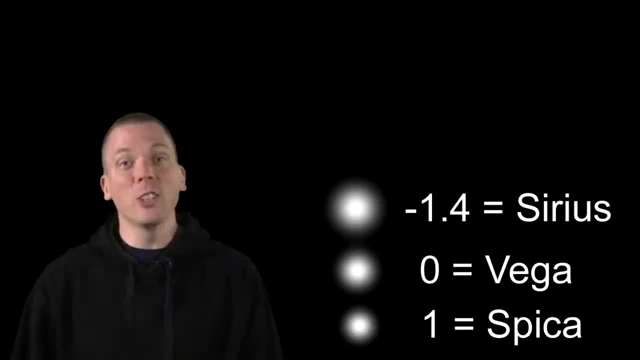 brighter than most other bright stars and it shines at magnitude negative 1.4.. The planet Jupiter is even brighter than that, often appearing at around magnitude negative 2. And Venus brighter still, typically around negative 4.. When objects are bright, they. 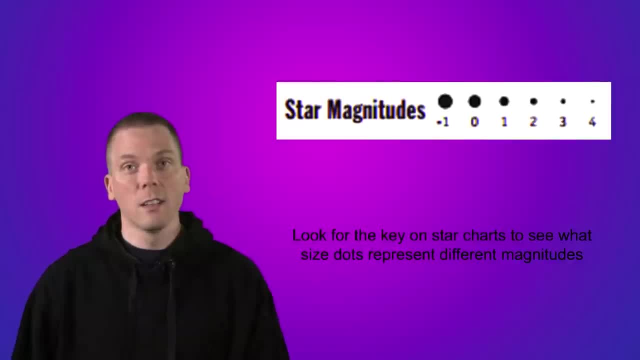 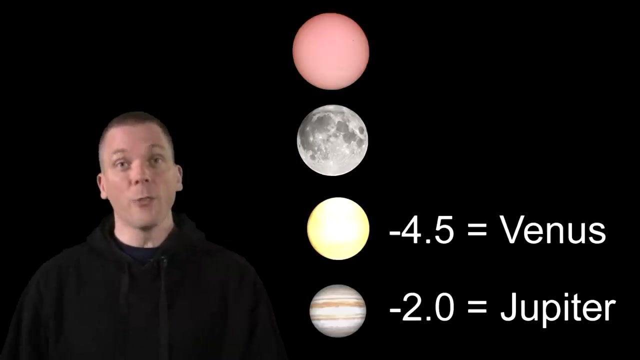 are denoted on star charts with larger dots. Dimmer stars are usually given smaller dots. This helps us locate brighter objects in the sky more easily, But from our perspective, even brighter than the stars' magnitudes is that of the moon and sun. The full moon in the night sky shines at magnitude negative 12.7, and the sun at 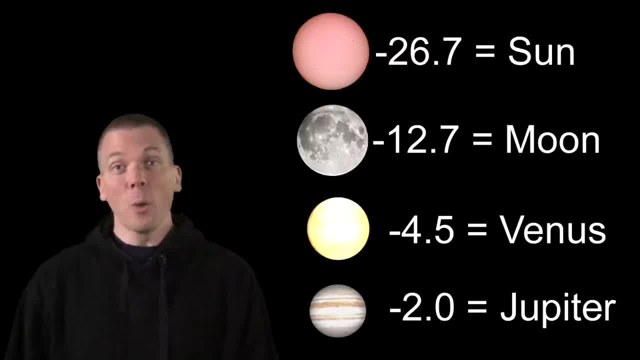 magnitude negative 23.7.. Those are both really bright compared to starlight, but also a huge difference even between themselves, as the sun is 400,000 times brighter than the full moon. Everything we have discussed has been visual magnitude, meaning how bright or dim objects 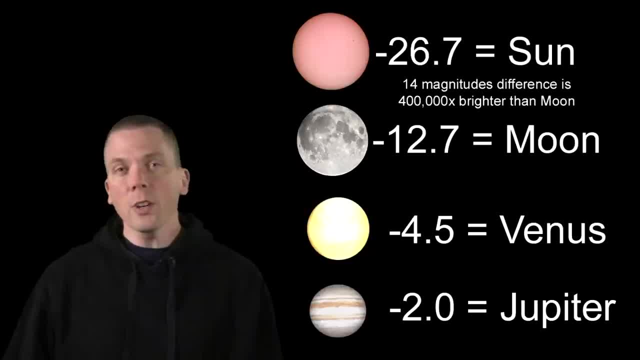 appear from our location right here on Earth. Another concept that you may run across is absolute magnitude, used by astronomers to compare the relative brightness of the sun to the absolute magnitude of the moon. The absolute magnitude of the moon is the absolute magnitude of the moon, The absolute 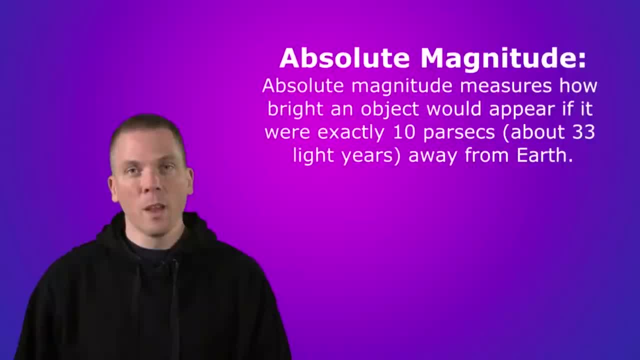 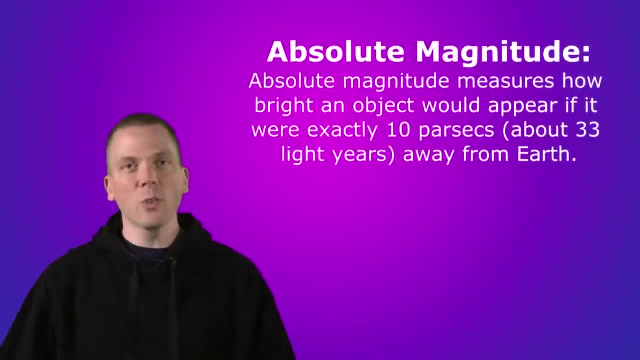 magnitude of the moon is the relative brightness of objects when placed the same distance, But that's a little more complex than what we need to know for simple stargazing purposes. All you need to know about it is that it compares the relative brightness of objects if they 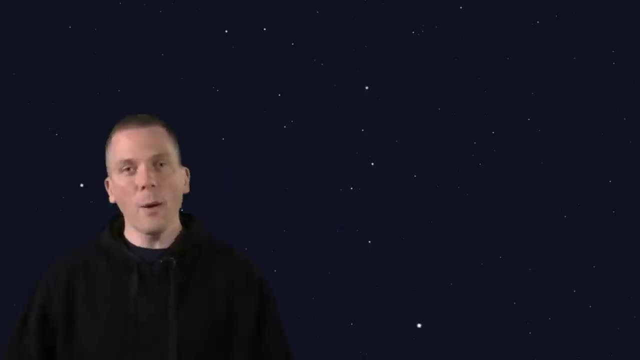 were all viewed from the same distance away. However, for visual magnitude, it helps to understand how it relates to other objects besides stars. Stars are point-like objects in the sky, so it's easy to assess their magnitude and brightness. Star clusters and nebulae are not quite as simple, so we look at their integrated magnitude. 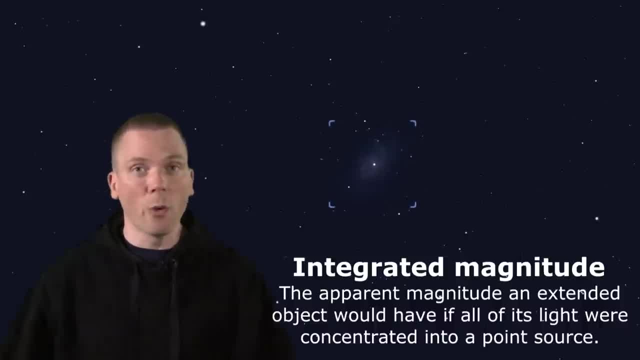 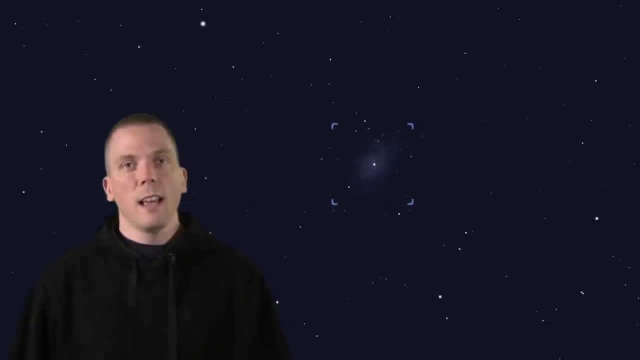 That's a way of saying that the same magnitude is now spread out over a larger area. For small objects, that can mean it is something that will look brighter to us in telescopes. If the area is very large, though, such as the galaxy M33 or the nebula M1,, these objects 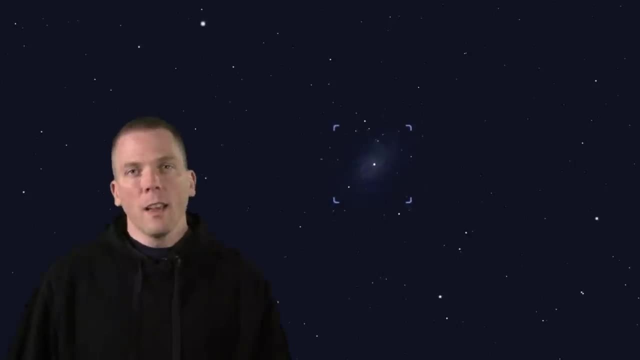 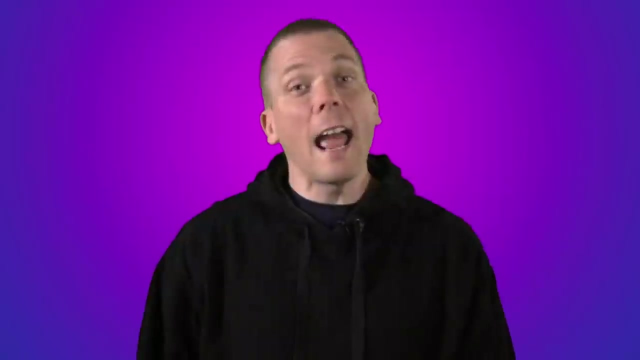 may look very dim, relatively speaking. If possible, try to look for the surface brightness of an object. Objects above a surface brightness of 11 or 12 can be very difficult to find, particularly from light-polluted areas. That's a quick overview of the magnitude scale and how to understand it, Just remember. 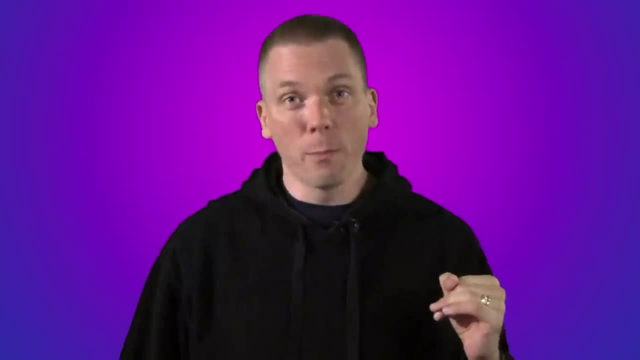 the Sun and Moon have negative magnitudes and are the brightest visual magnitude. objects and higher numbers are dimmer stars and objects. You'll be in good shape. In the next video I'll explain how to easily measure distance in the sky moving from bright. 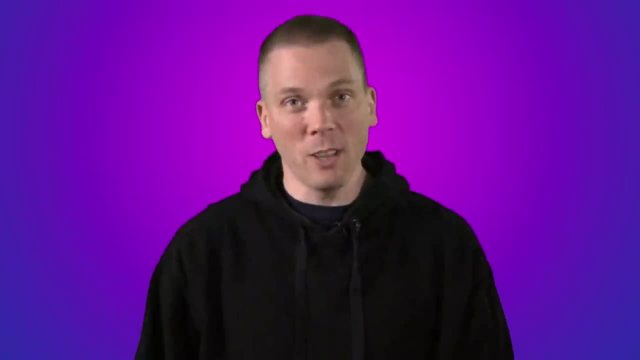 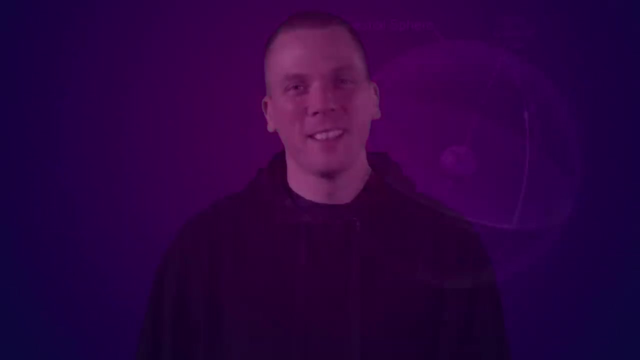 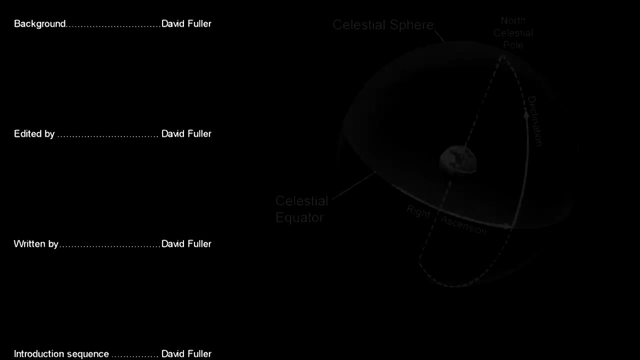 objects to the distance. Thanks for watching. I'm David Fuller. Keep your eyes on the sky and your outdoor lights aimed down by using dark, sky-friendly lighting fixtures so we can all see what's up. Subtitles by the Amaraorg community.